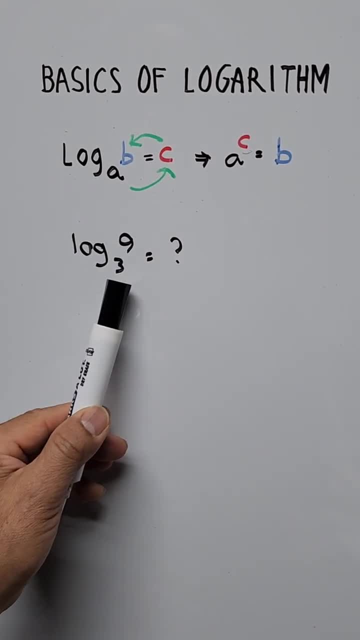 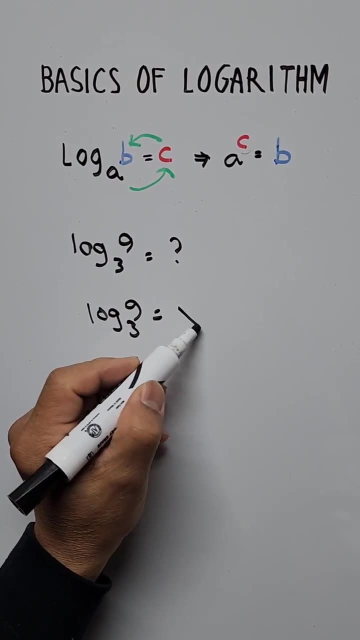 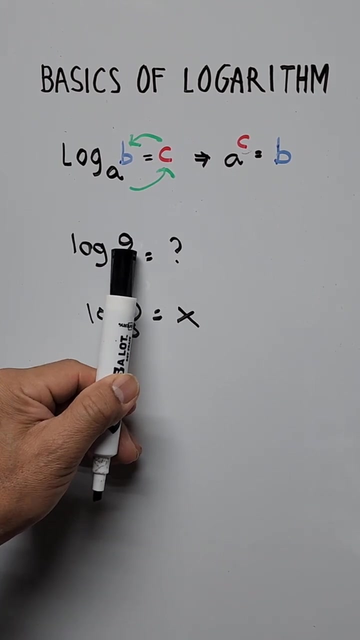 Here are the basics of logarithm. Logarithm of 9 base 3 is what? So this is: log of 9 to base 3 equals x. So this logarithmic expression asks which exponent of 3 equals 9.. So we have here now x. 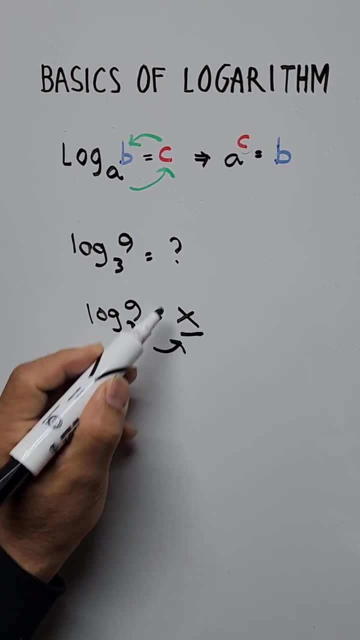 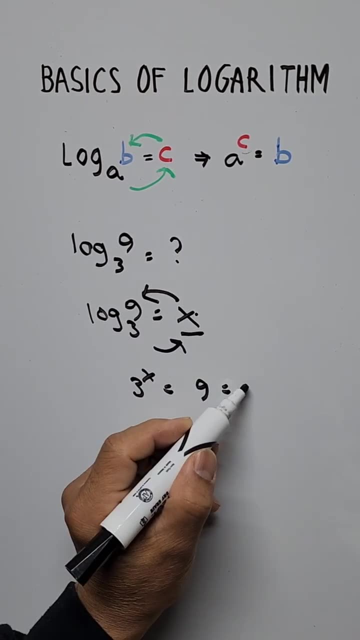 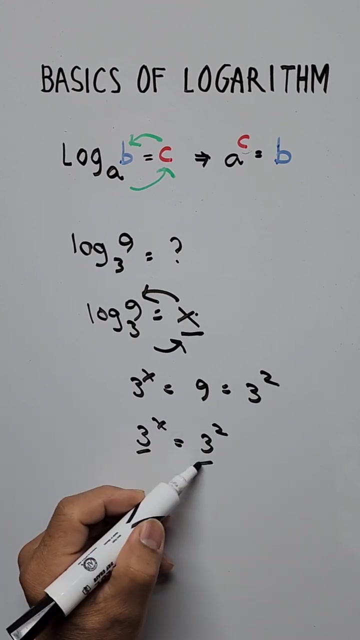 is the exponent. So this follows a pattern. So 3 to the power of x equals 9, and 9 can be written as 3 squared. So 3 to the power of x is equals to 3 squared. They have the same base. This means: 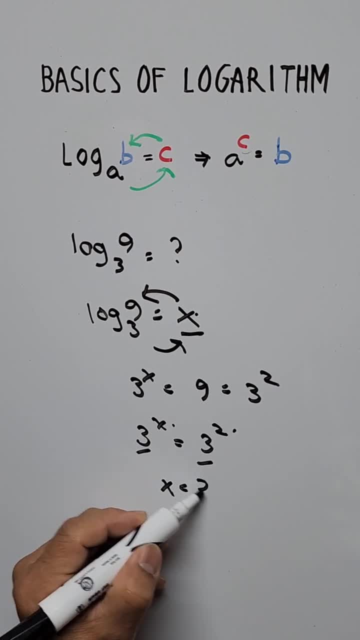 their exponents must be the same, So x is equal to 2.. That is our answer.